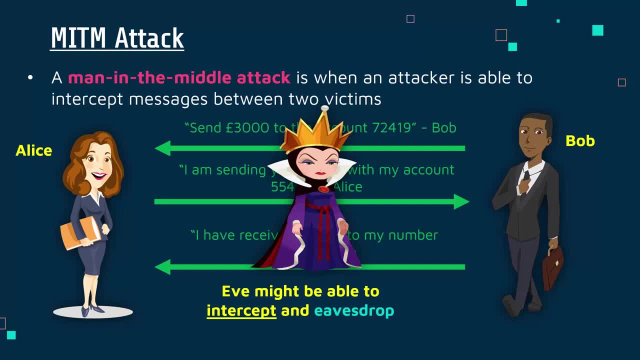 in a cafe and can intercept their Wi-Fi, or maybe she's managing to hack into a router and can intercept it. She's finding some way to listen into our messages here, And so, with this information, she knows that Alice is going to be intercepting the messages and she's going to 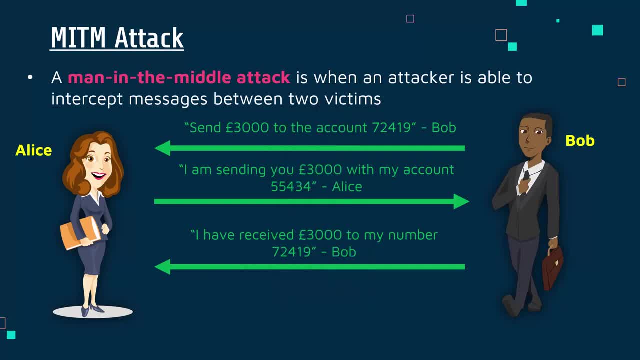 know that Alice has got a lot of money and now Bob has got the money. Maybe she's able to take their bank account details and cost them some money in that way and extract money from them. But this is just eavesdropping. Eavesdropping is its own attack, really, where we're just listening. 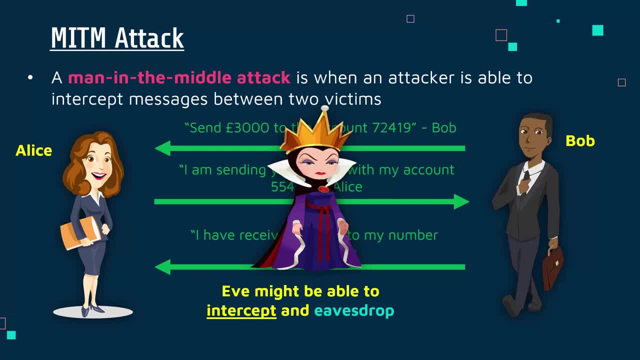 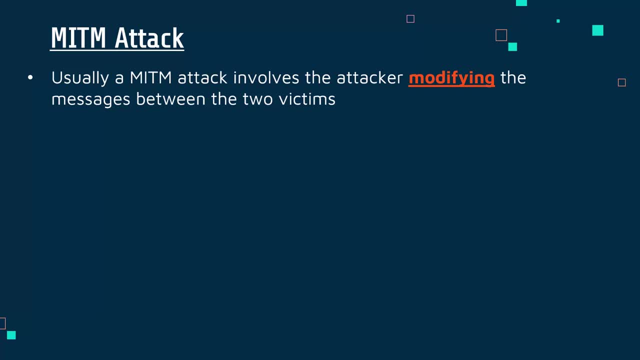 in. We're not actually doing anything, And usually a man-informed attack is a bit more active than this. Usually, we're actually going to, as an attacker, going to actually modify the messages between the two victims. Eve was not doing anything, She was just listening to it, which is 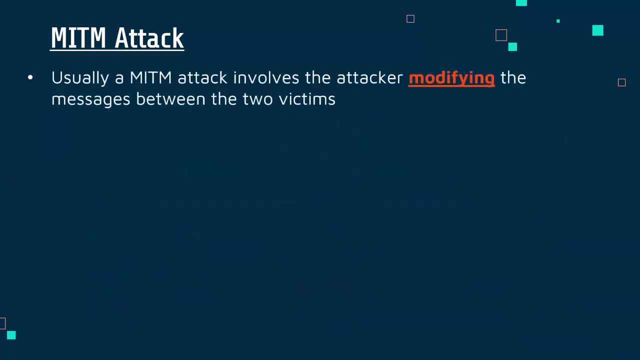 still illegal, but she was listening to it, Whereas normally an MITM attack is actually modifying the messages, and this can take it to a slightly more extreme level. So let's use the same scenario again of Alice and Bob. Alice is trying. 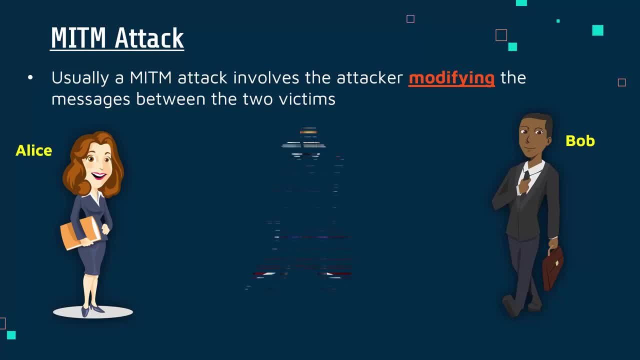 to send some money to Bob. He's trying to receive money from Alice. But this time, let's say we've got an actual man here. Let's say we've got Mallory, who is our person, who is our attacker, in the middle of Alice and Bob. This time he's able to actually intercept and stop messages. 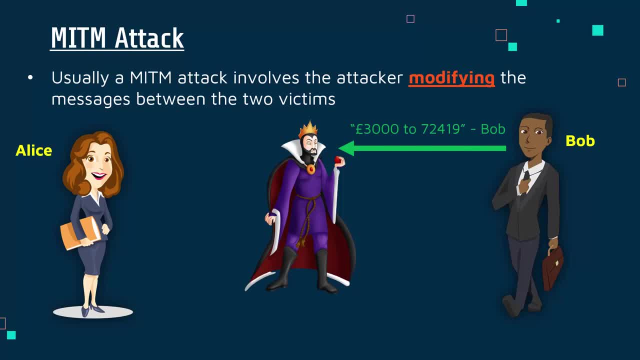 coming from Bob. So the first message requesting three thousand pounds to his bank account is being taken by Mallory, not Alice. Bob doesn't know that the message is not going to Alice. He thinks it's gone to Alice, but actually Mallory has managed to intercept it. Now here he might actually manage to. 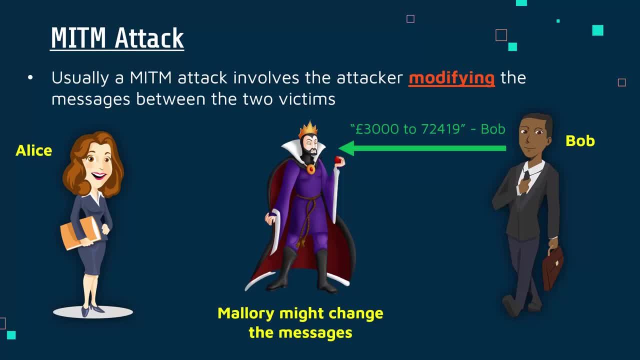 change the message. So instead of saying it's going to account number 7419, he might change it So it's going to 18845, which let's assume is Mallory's bank account. Alice receives it thinking it's. 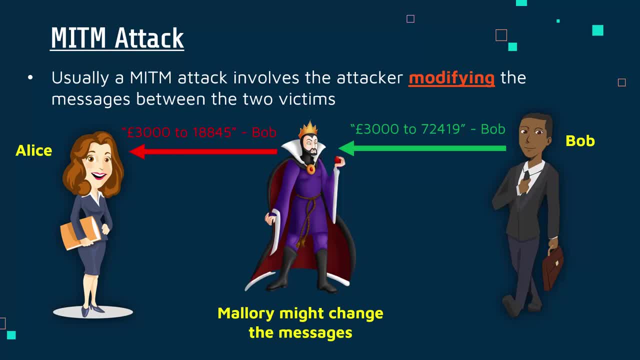 coming from Bob. She's got no idea. we've got Mallory in between changing his message. So Alice is going to send a message to who she thinks is Bob but actually is Mallory, And so maybe Mallory does nothing, Maybe just ignores it and moves on. Maybe he sends a message to Bob saying: okay, sorry. 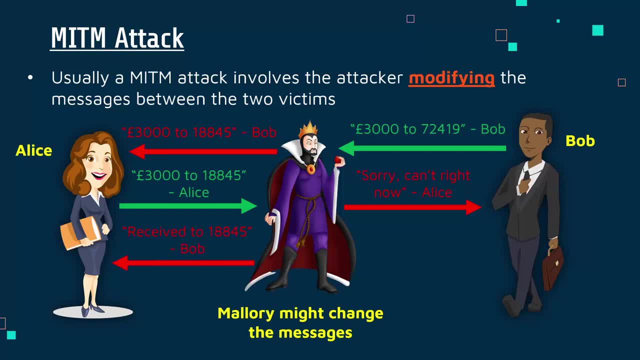 I can't right now. And Bob thinks: but actually that's coming from Alice. He doesn't realise that actually money is never going to arrive because Alice has sent it to the wrong person. But then Mallory might try and convince Alice that things are all okay by sending a message from Bob. It's